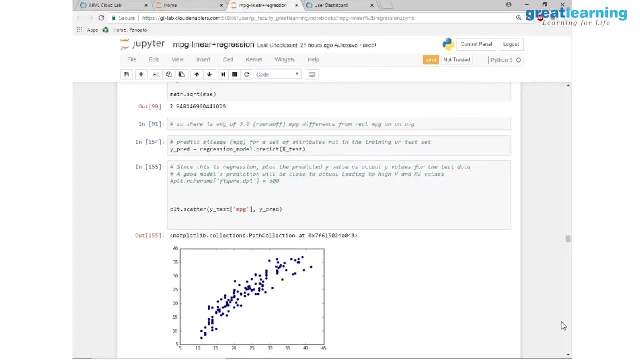 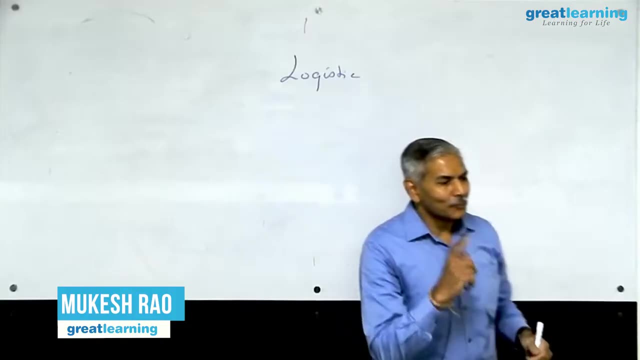 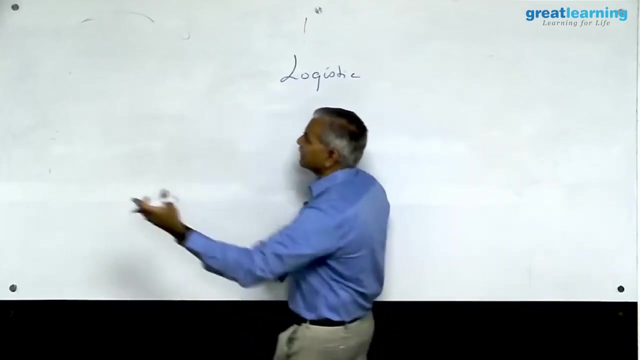 I would like to take you on to another important model, another important, very commonly used model, which is called the logistic regression. One homework I would like to give you is in linear models. we never implement linear models in production. What we implement is a variant. 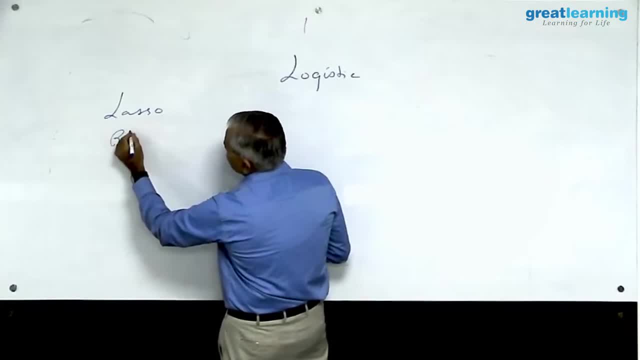 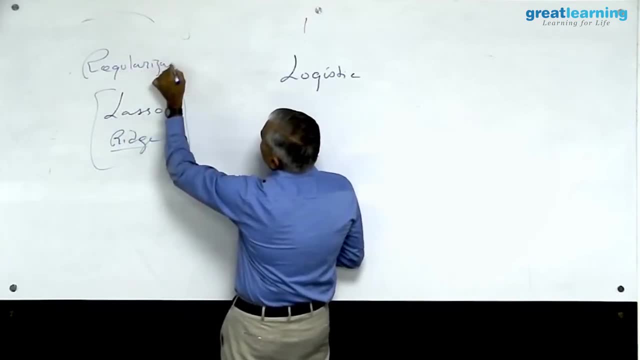 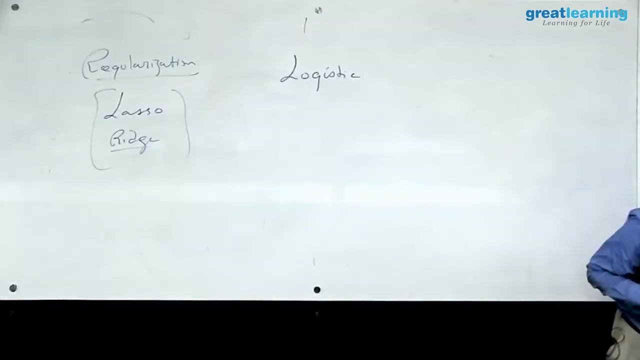 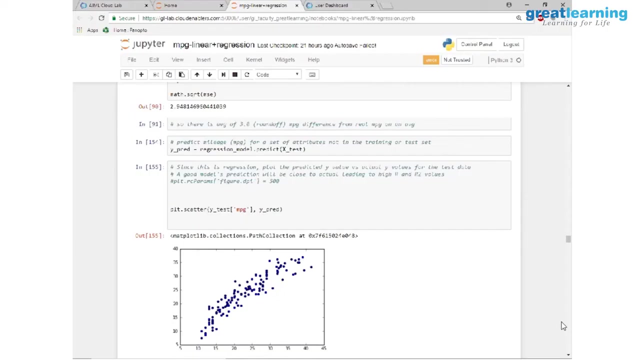 of that which is called lasso or ridge, These two techniques. they go under the name of regularization. They are called. all models are actually regularized. Regularization is a way of controlling the behavior of the algorithms which are creating these models. for you, Regularization. 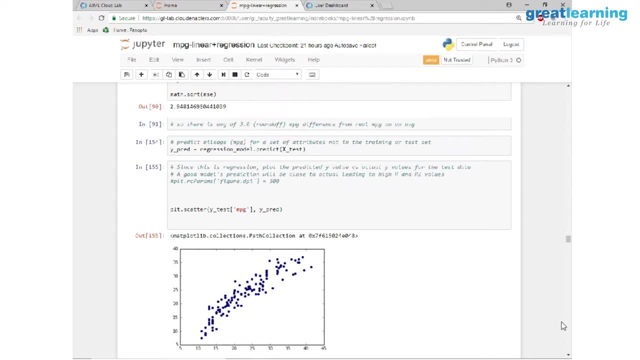 helps you to prevent you from getting into over fit zone, getting into very complex models. What I would advise you to do is just go and read about them. You may not be able to grasp the whole thing unless you have a prior experience in all these things. You may not. 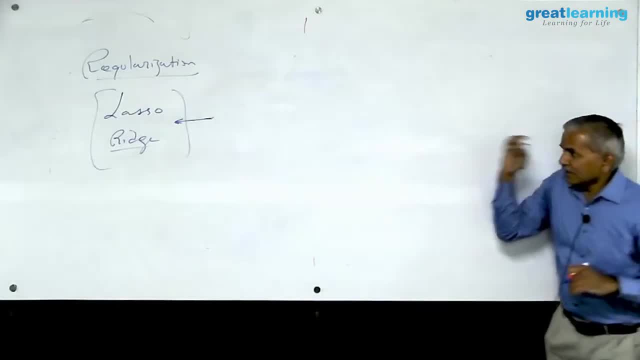 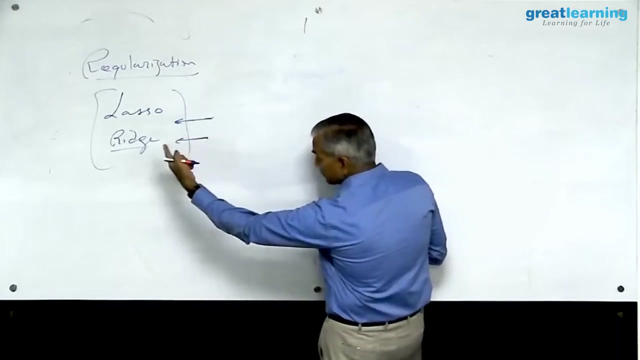 be able to grasp lasso and ridge. So what we implement is one of these two. Both of them are linear models with what we call the thing regularization. Ridge regression helps you to eliminate unnecessary dimensions. It is also used for dimensionality. 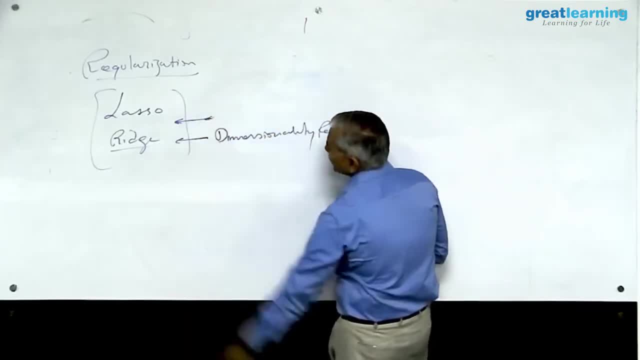 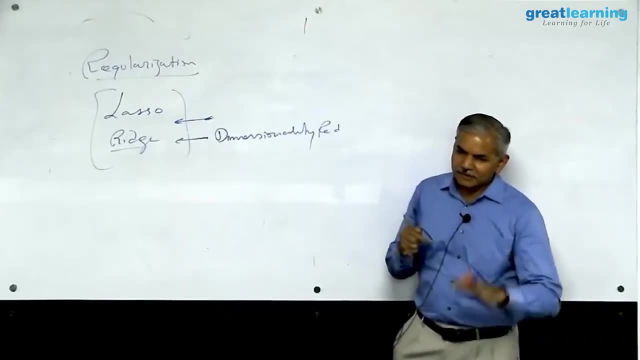 reduction. This one does not eliminate any dimensions, but it makes the whole thing recorded, educated. Jae hae them almost close to useless dimension, Any useless dimensions. it tries to suppress the influence of the useless dimension on the target by converting the coefficients very close to 0, but it does not make them. 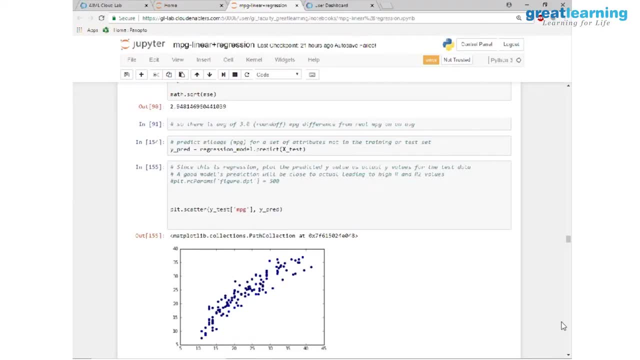 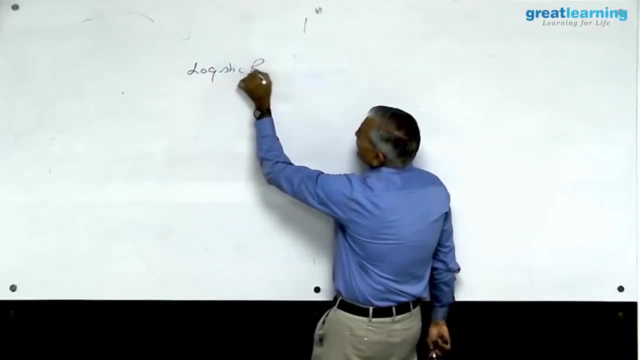 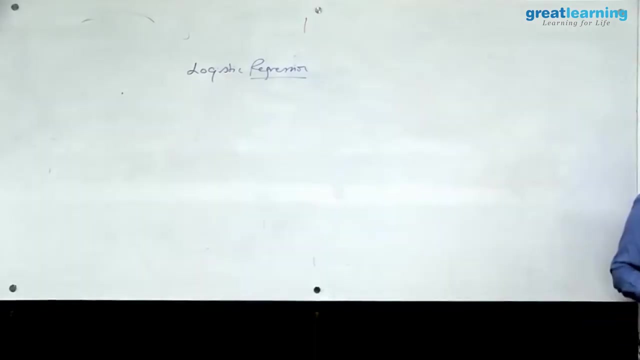 0.. Now I am going to take you to a technique, a model algorithm called logistic regression. We call it logistic regression. The word regression is misleading here. you are not going to predict any values, you are going to do classification. 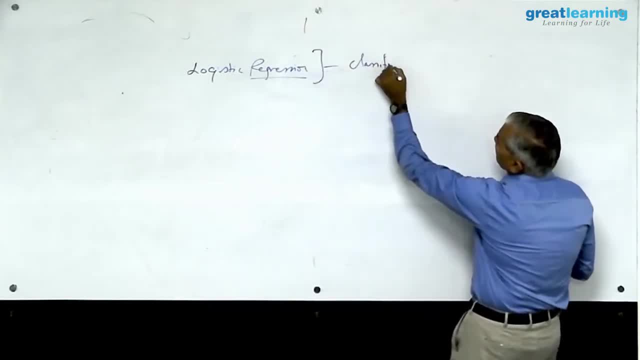 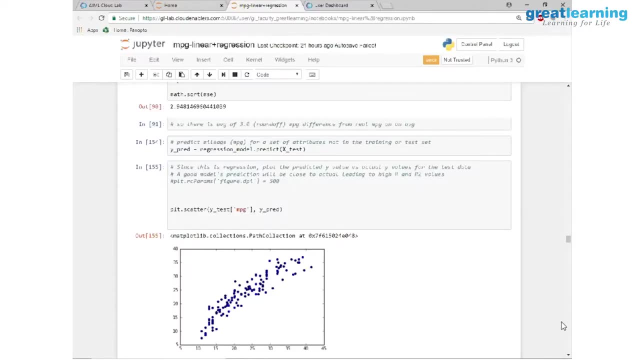 This is only for classifications. it is not for predictions. The reason the word regression is used is underneath this algorithm. underneath this model is actually a linear model. that is why it is called that. Now, imagine you are working in a bank, you are a data scientist in a bank and your management 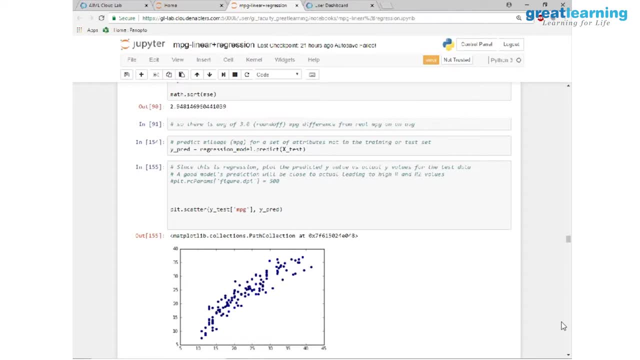 has asked you to come out with a model which will help you to predict whether a person who is applying for a loan Is he likely to become a defaulter or a good customer. Will he return the loan or will he be a defaulter? 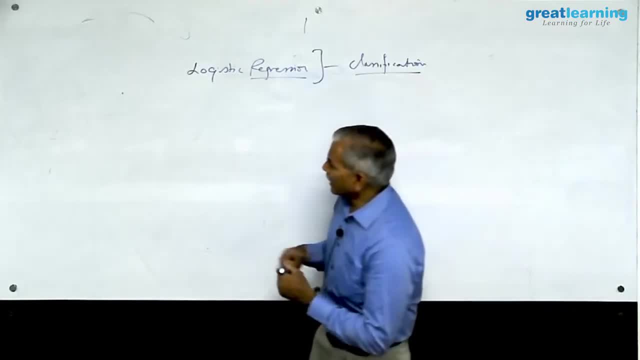 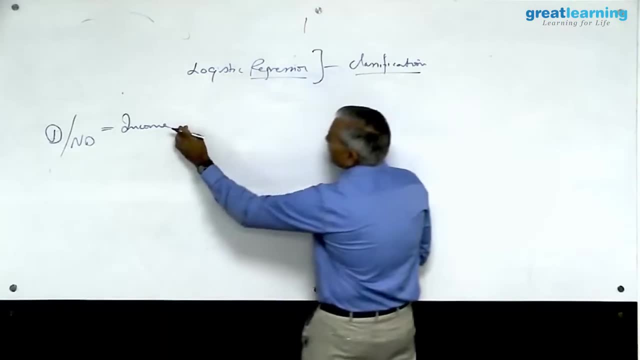 So you have to build a model for that. So can you tell me some of the attributes that you would like to collect, which will help you to predict whether it is going to be a defaulter or a non-defaulter? Income expenditure, blah, blah, blah, blah, right. 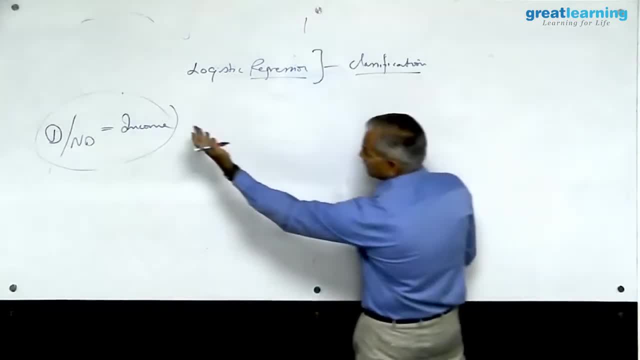 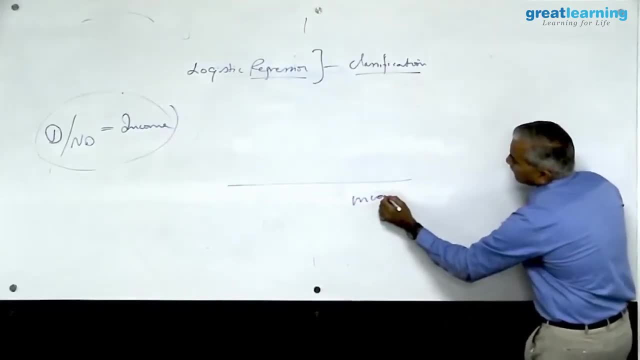 Let's take one simple case of income. So of course it also depends on various other parameters: loan amount, loan duration, blah, blah blah. So let's take only income part. Okay, On this income part, amongst other dimensions that you have on this income part, when you 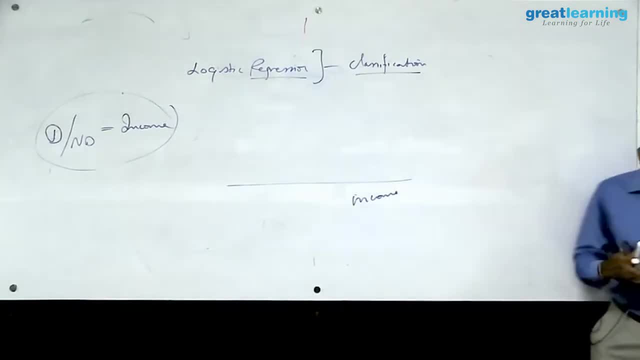 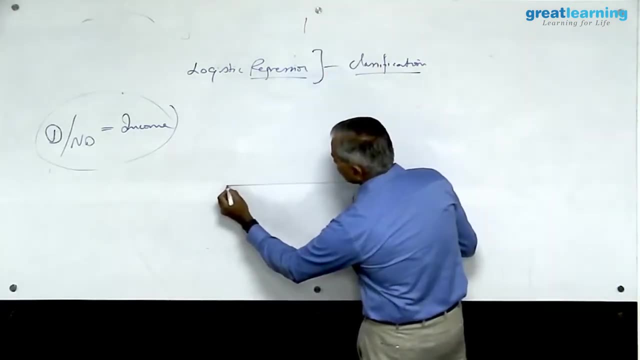 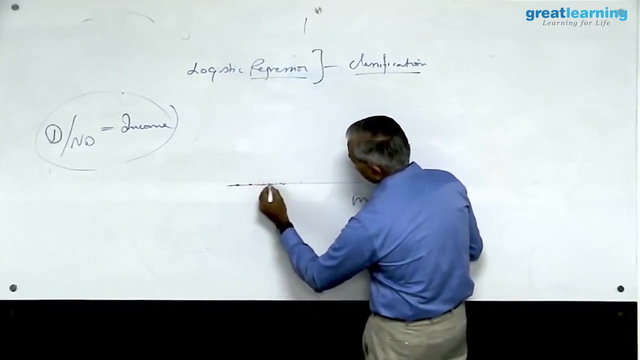 do an analysis of this, you find a very interesting pattern, And the pattern is the defaulters are generally, you know, on the lower income side. the defaulters you find are on lower income side, defaulters indicated by red. And as you go towards higher income side, the density of defaulter falls, which actually 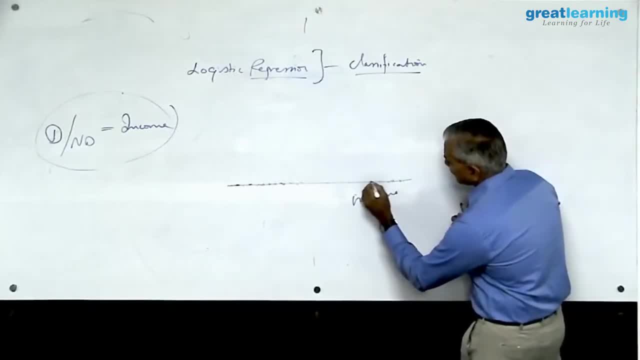 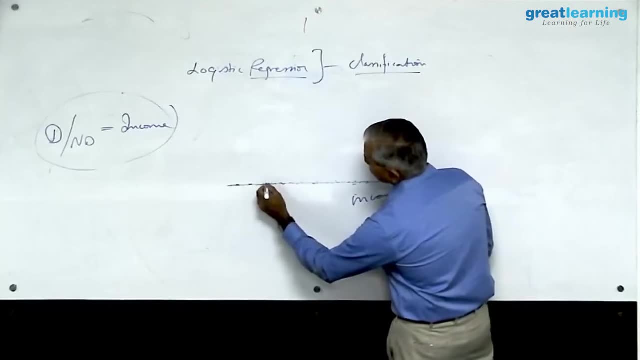 in reality is opposite All high income groups. you see a lot of good customers here, okay, a lot of people who return their loan on time, so on and so forth, But you also see them here. It's not that they are completely gone, but you also see them here. 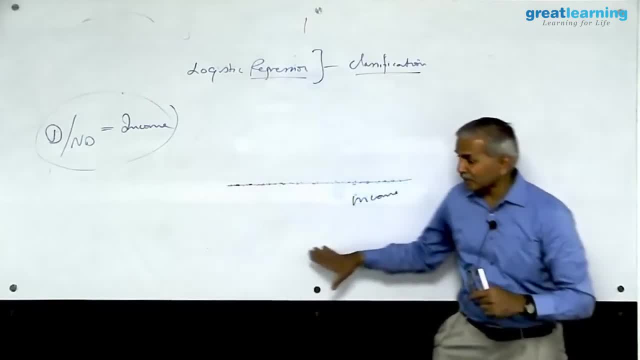 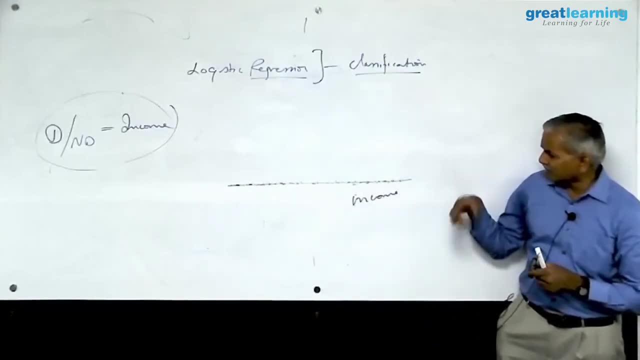 So I have taken one attribute. there are many attributes. I am studying just one attribute. On this one attribute, I am finding that more defaulters are concentrated towards lower income side, very few on the higher income side. more non-defaulters are on the higher. 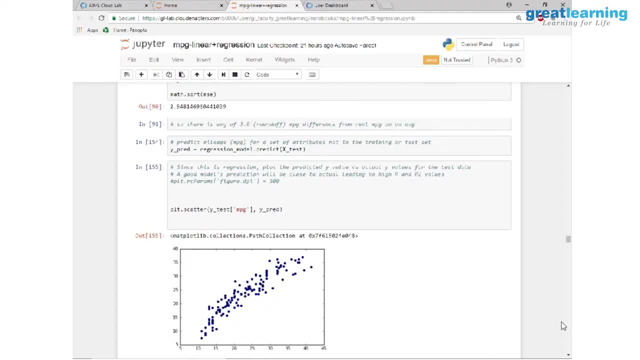 income side and very few of them on the lower- Okay, Lower- income side. Now I want to convert this pattern which I am seeing in my data, some kind of clustering which I am seeing in the data. I told you, patterns means clusters also. 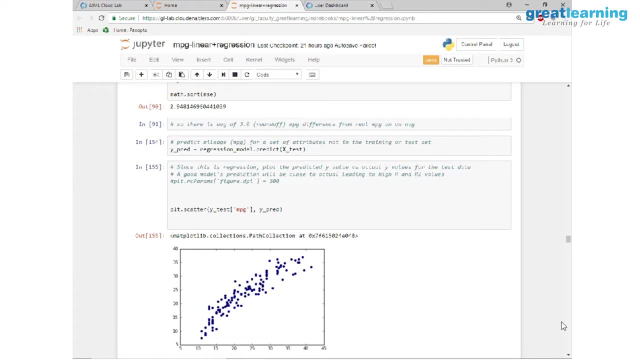 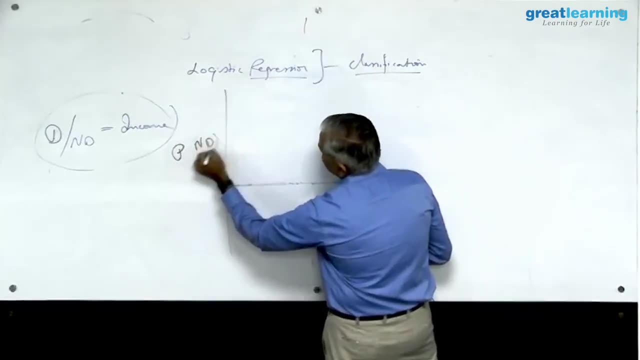 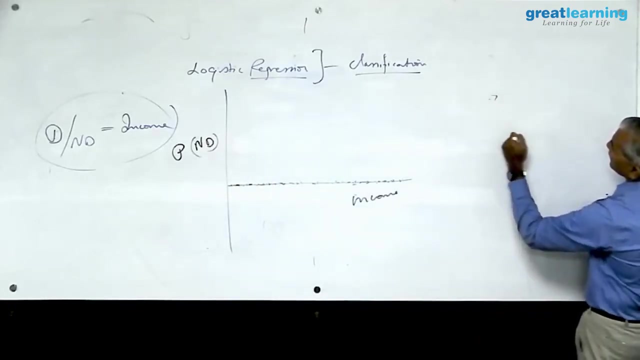 I want to make use of this and build my model. I say, okay, let me build a model where this axis represents probability of non-defaulter. You could have taken a defaulter, also non-defaulter. So if probability of somebody being non-defaulter is 0.7, then probability of him being defaulter. 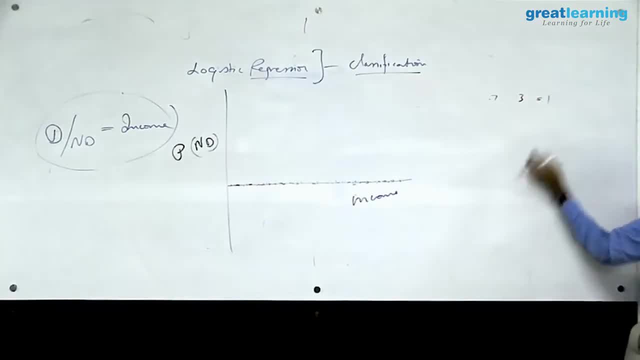 will be 0.3.. Because probability has to come to 1.. Okay, So you can take any class. I am taking non-defaulter and the other thing which I do here is: all the non-defaulters, I am going to encode them as 1, all the defaulters, I am going to encode them as 0.. 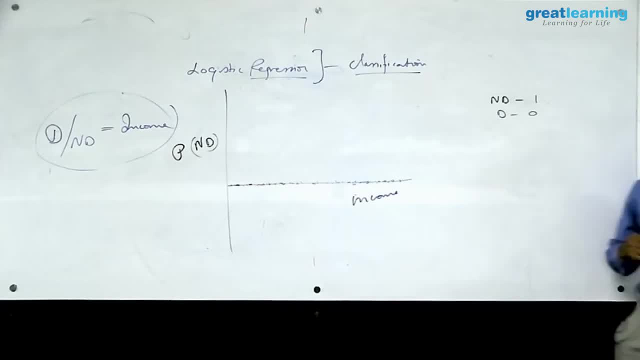 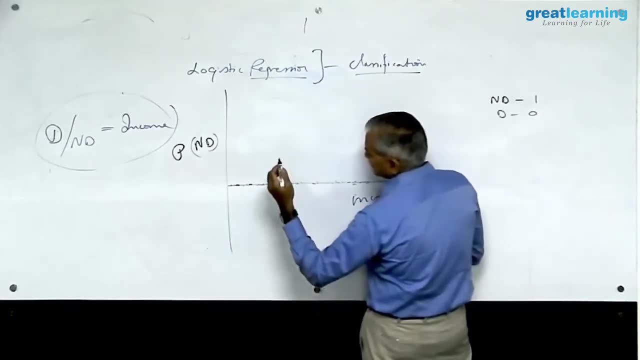 Once again, it does not have to be this way, it can be the other way also. Now, when I do this, what this model- linear model- tells me is what the linear model which I built on this It tells me is. 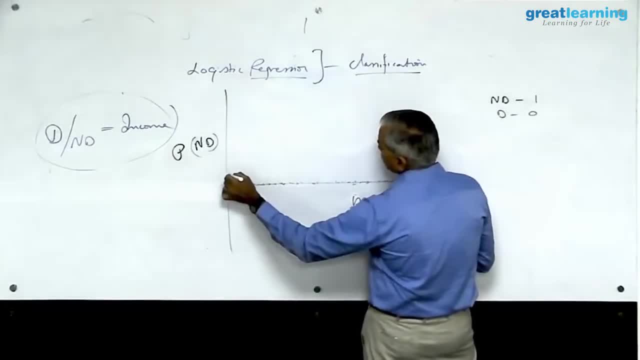 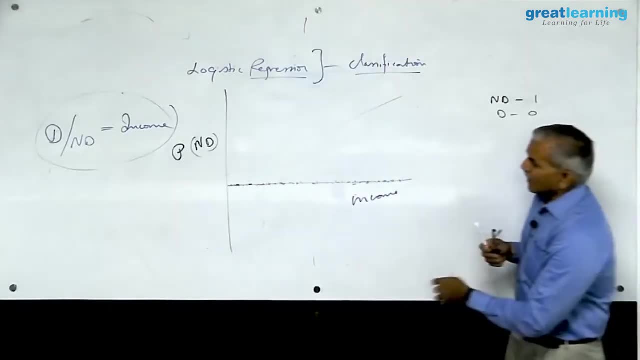 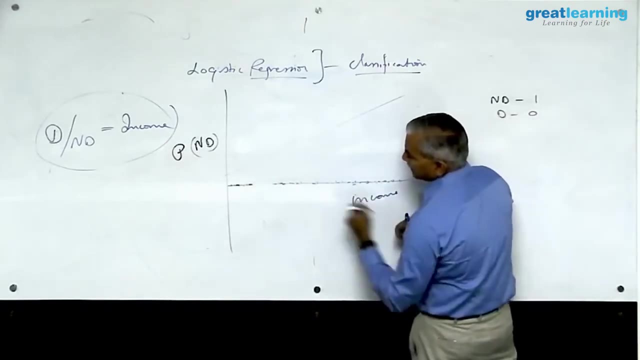 As you, As the income increases, probability of that person being non-defaulter increases. That is what we are observing in this cluster. As the income increases, probability of any person being non-defaulter increases. As the income decreases, probability of person being non-defaulter increases. 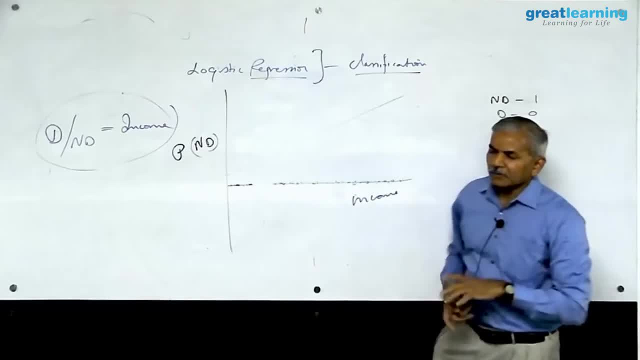 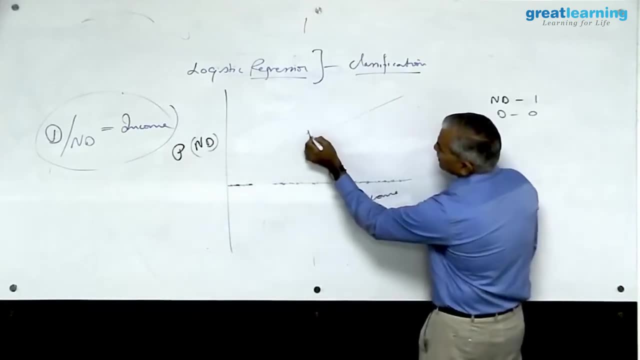 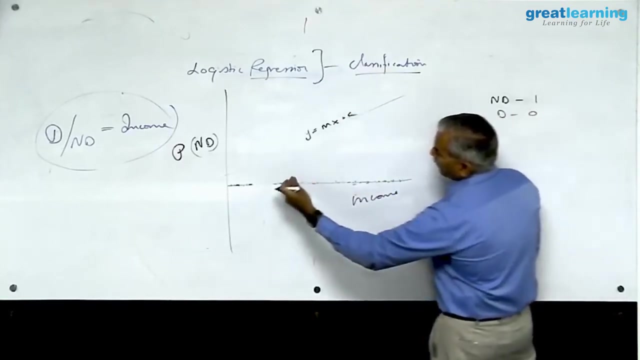 That is what we are seeing here. So this I want to convert into linear model. So when I do that, I get this line. Okay, This line, This line is of the form y, equal to mx plus c, where x is your income and m is the slope. 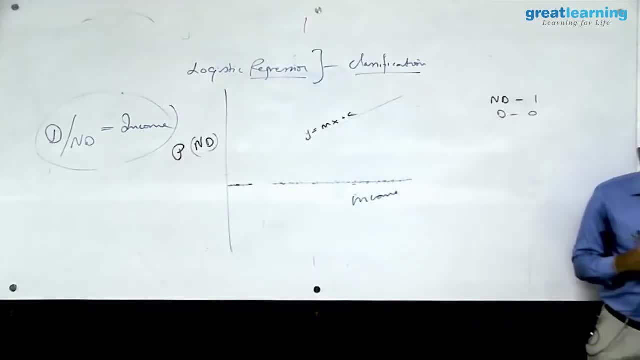 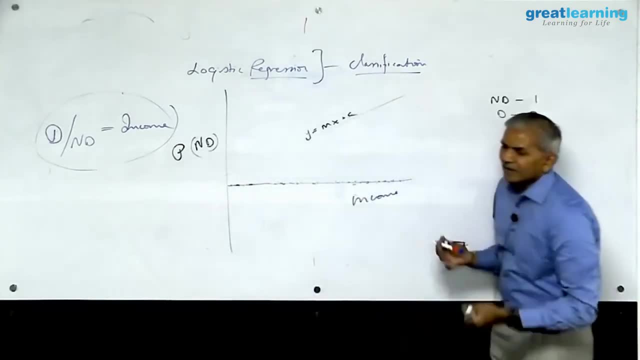 of this line with the horizontal axis. But the problem of this approach is your probability model. a line goes to infinity, from minus infinity to plus infinity. So, but probability cannot be infinity. right, Line goes from minus infinity to plus infinity. In fact, it cannot even be 0, it cannot even be 1.. 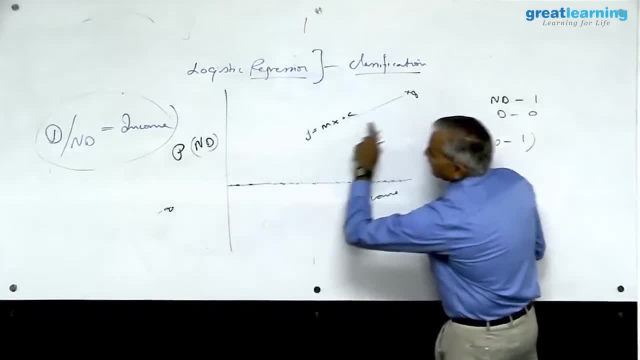 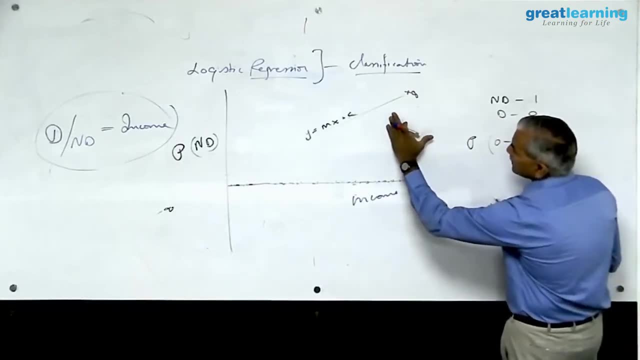 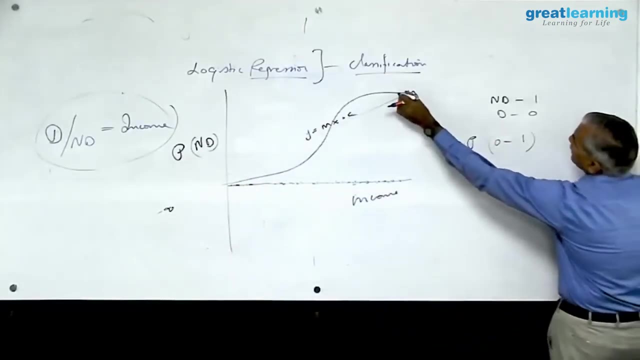 Probability is always in between. So the line does not help us Because it can go beyond to infinity minus infinity, both sides. So what we do is we convert this line into an S-curve, where the S-curve is called the. 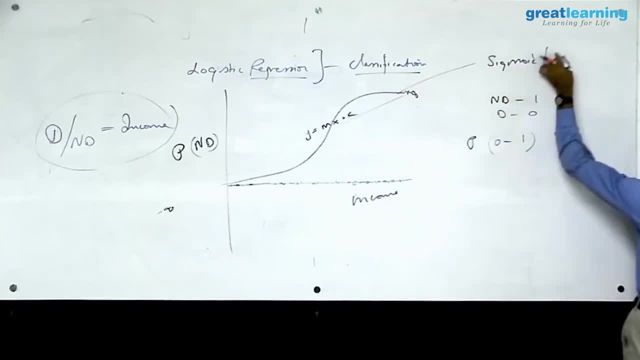 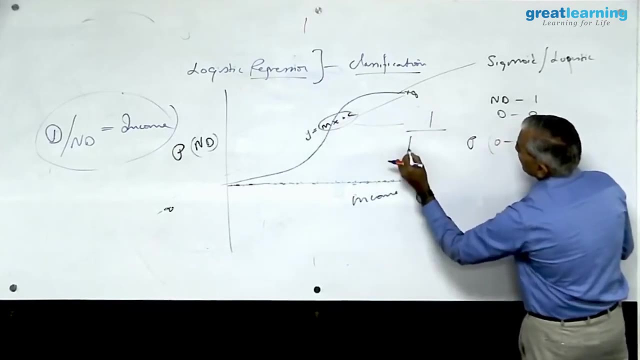 sigmoid curve also goes with the name logistic. How do you convert this into a S-curve? How do you convert this into a S-curve? How do you convert this into a S-curve? You feed this y equal to mx, plus this expression. you feed into an equation: e power minus mx. 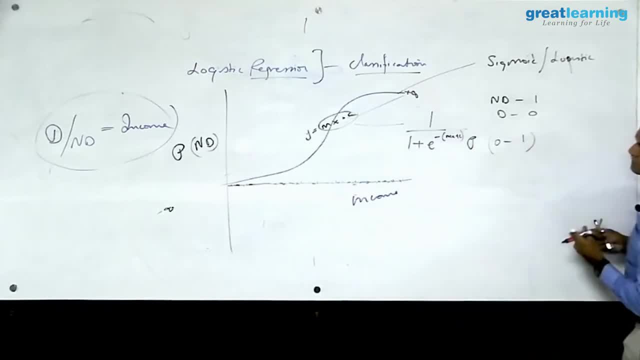 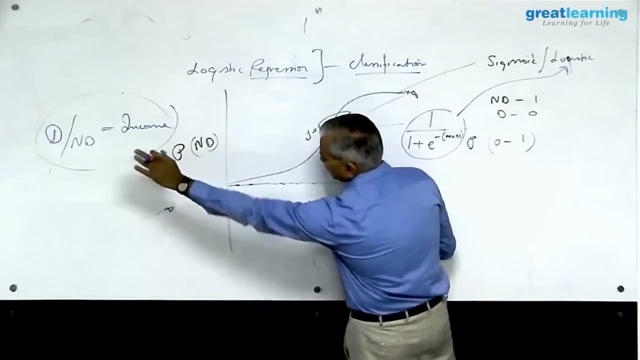 plus c. This function is called, some people called it logit, some people call it logistic function. This function has a beautiful property. The property is it goes towards 0 and becomes 0 at, only at, infinity. So it never becomes 0 for all practical reason.